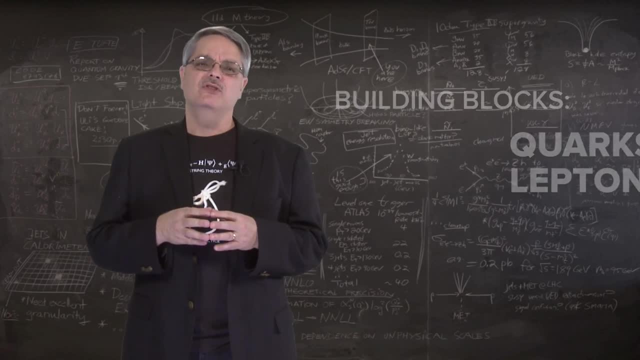 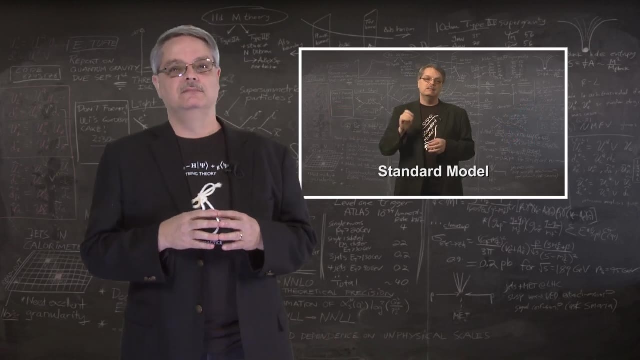 between the quarks and the leptons. The name we have for this model is called the Standard Model of Particle Physics, and if you want to know more about it, I made a video that gives a bunch more details. The problem is that if we want to get at the ultimate building blocks of the universe, 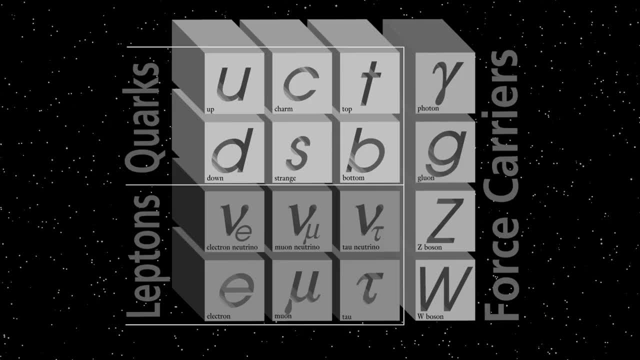 what we currently know doesn't seem to completely fit the question. If we want to get at the ultimate building blocks of the universe, what we currently know doesn't seem to completely fit the question. We have six types of quarks: three charged leptons, three neutral ones. 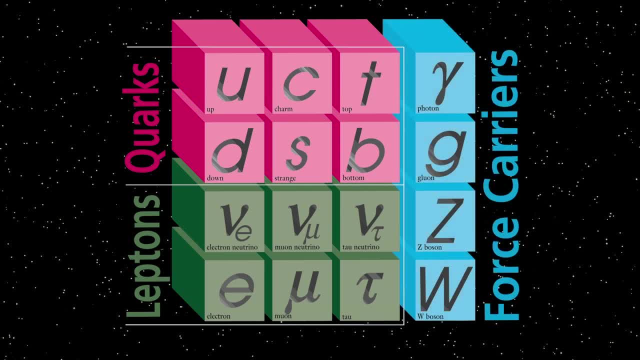 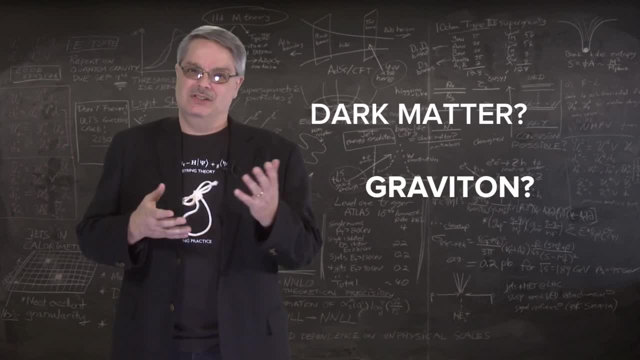 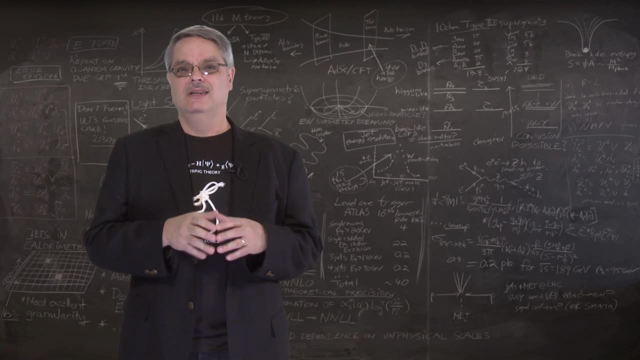 and four force-carrying particles. Plus, when you include the mysterious world of dark matter and a so far undiscovered particle called a graviton, the situation is a ridiculous mess. Some have charge, some don't. Some particles feel some forces, but not others. 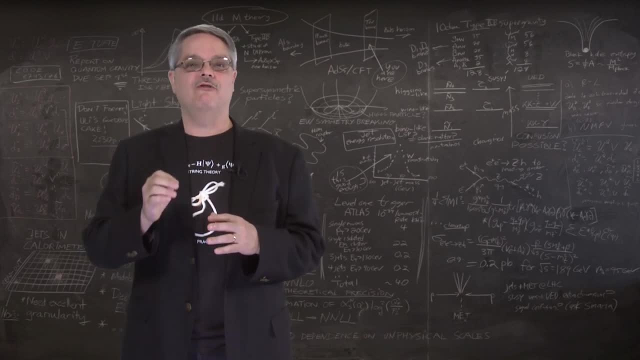 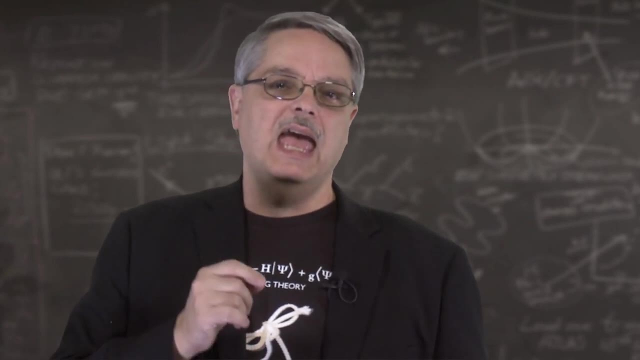 It's hard to imagine that the ultimate building blocks and most fundamental rules are found in this complexity. It seems there must be something simpler underlying all of this. As we dive into the world of the super-small, we encounter molecules, then atoms, then protons. 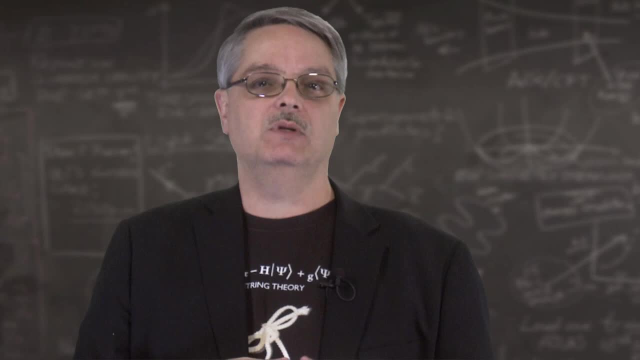 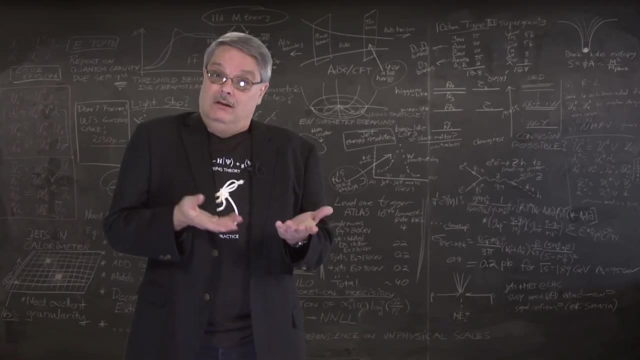 neutrons and electrons. Digging deeper, we find quarks and leptons. So could there be another layer, Or two, Or three? Well, sure, Even though they haven't been found and, to be honest, may not even exist. 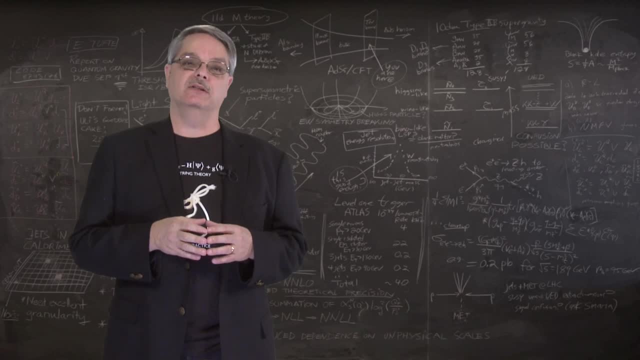 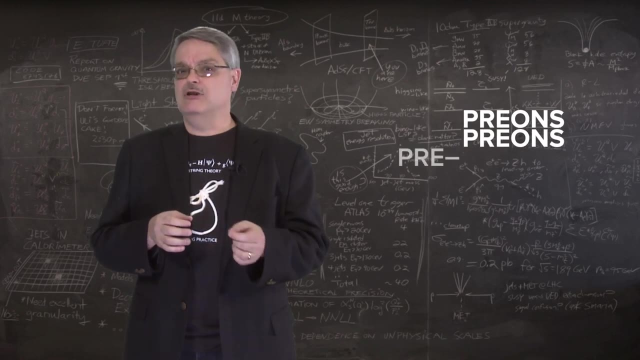 we already have a name for the layer below the super-small. The layer below the super-small is called the electron layer, And that's why we have quarks and leptons. These smaller particles are called prions. But there's no reason there couldn't be preprions and prepreprions and so forth. 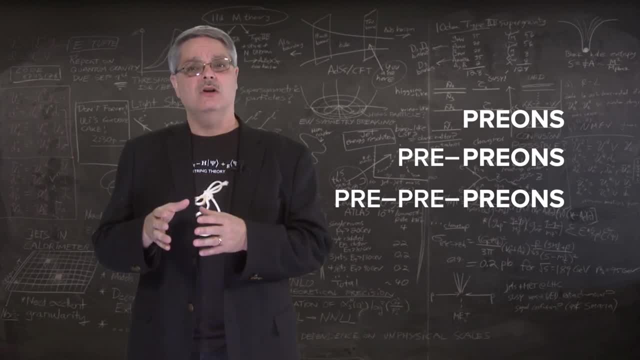 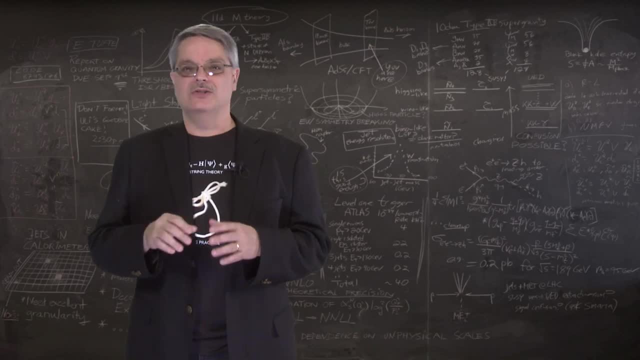 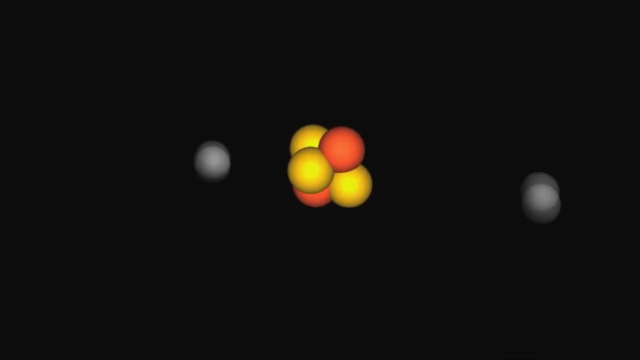 In short, there could be a long line of undiscovered particles before we find the ultimate and smallest particle of all. This seemingly endless ladder of particles isn't the only idea out there. One very interesting idea is that when we get to the smallest size of all, we don't 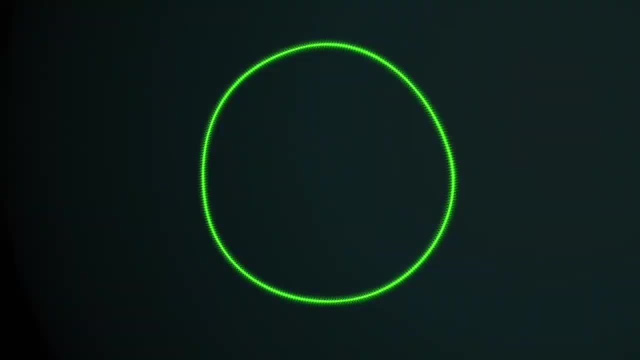 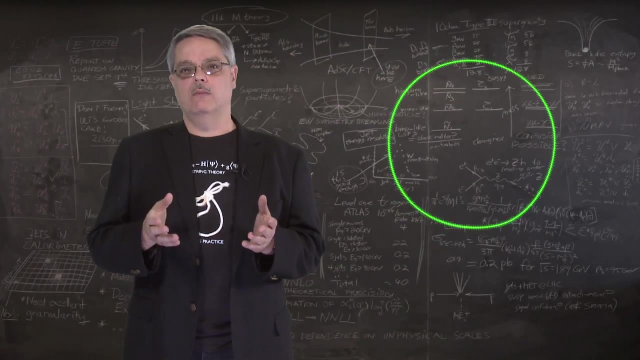 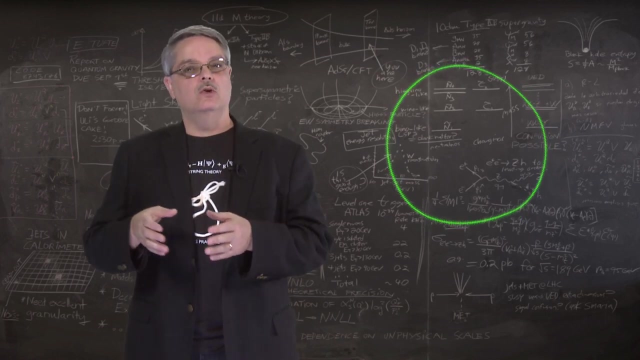 find a particle, but rather an ultra-tiny vibrating string. So how does that work? How can a string explain the variety of subatomic particles we know about? Essentially, scientists assign the various different vibrational patterns of the string to be the various known particles. 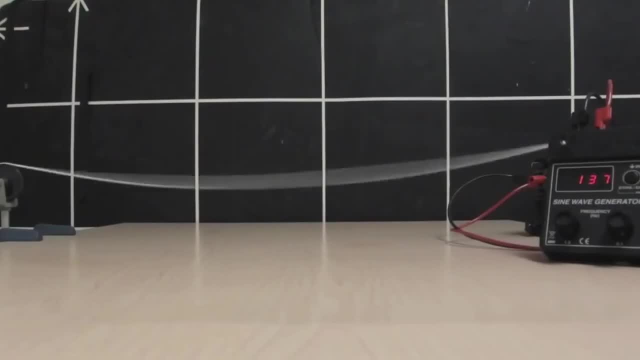 You can get a sense of this by seeing what happens with a single string. If you vibrate a string slowly, it vibrates. You get a single big vibration. If the vibration is increased, you get two big vibrations. Increase the vibration more and you get three vibrations, and so on. 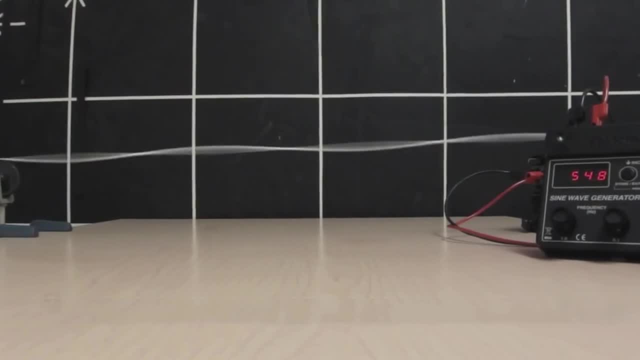 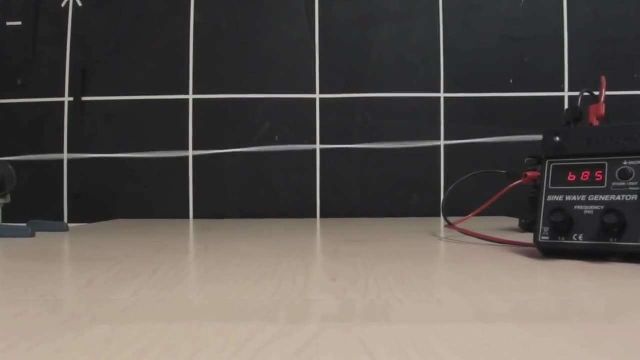 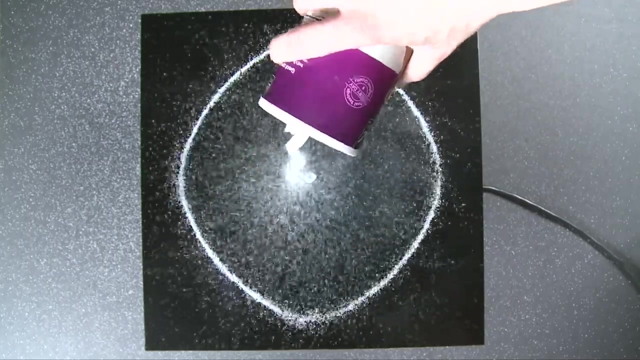 In the superstring model, each vibration pattern represents a specific subatomic particle. This is really cool because it means that all particle types originate from a single kind of string. The complexity of vibrations is even more obvious in two dimensions. Take some salt. 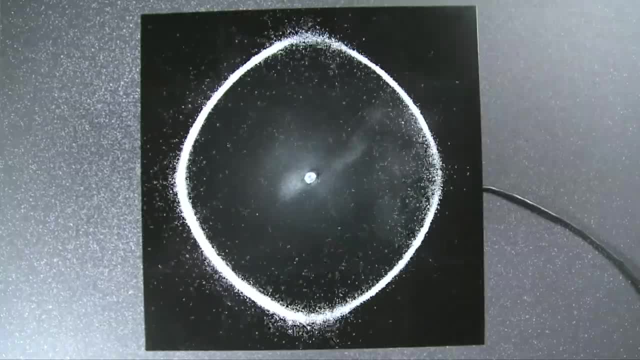 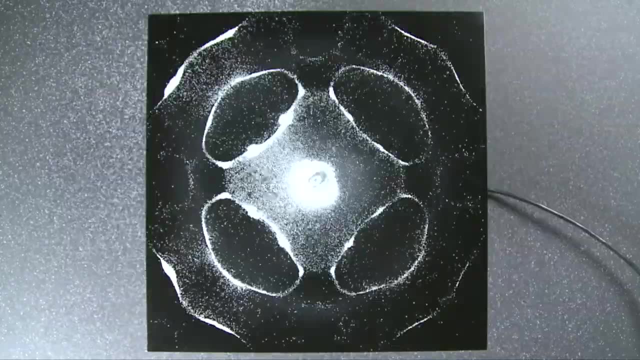 Put it on a metal plate And drive it with a speaker and remarkable patterns arise. In this example, the white lines are where the salt is stationary and the plates aren't moving. Where you see the metal of the plate, it's vibrating like mad, so no salt can sit there. 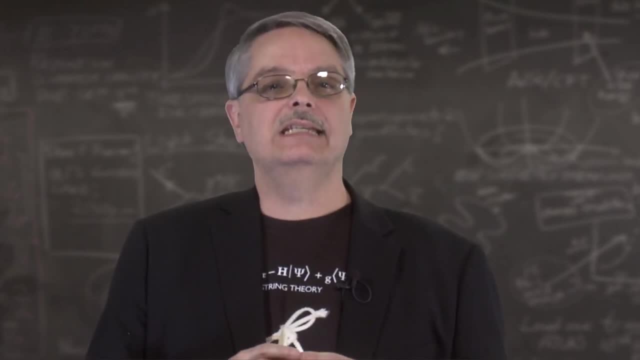 While two-dimensional vibrations are already pretty complex, scientists think that superstrings vibrate in way more dimensions, as in like seven dimensions. Yes, imagining more dimensions is hard to get your head around, but it's what the theory needs to work. The dimensions we're talking about here are much smaller than the ones you're familiar. 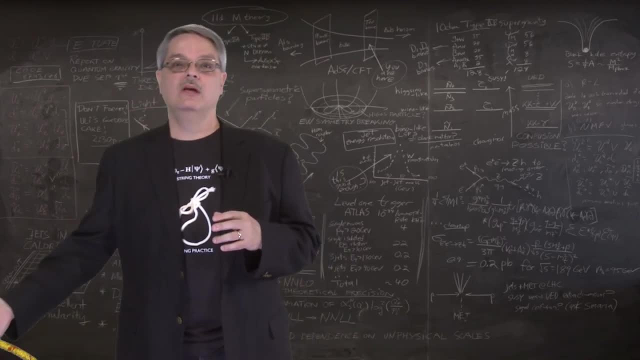 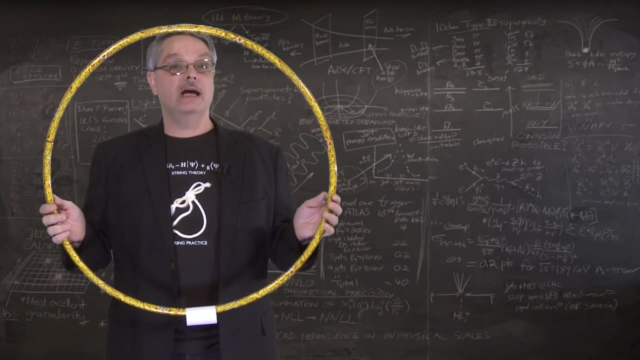 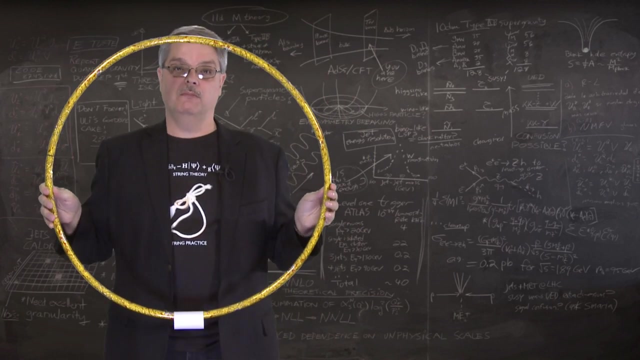 with. You can get your head around smaller dimensions using this hula hoop. The hula hoop can move in the familiar x, y and z dimensions of left and right, up and down and forward and backward. But you'll notice that the hoop has a little paper sleeve wrapped around it. If you want to explain the location of the piece of paper, one way to do this is to take a piece of paper and put it on the side of the hula hoop. If you want to explain the location of the piece of paper, one way to do this is to put 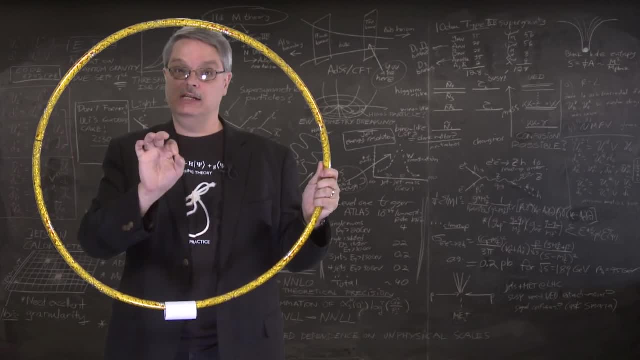 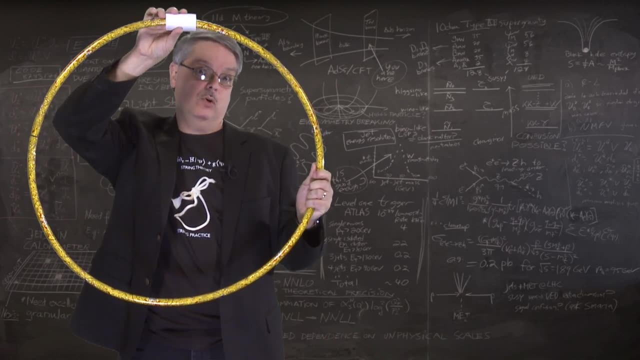 it on the side of the hula hoop. One way to do that is to locate the hoop center in x, y and z and then state the position of the paper on the hoop Bottom side, top and so on. 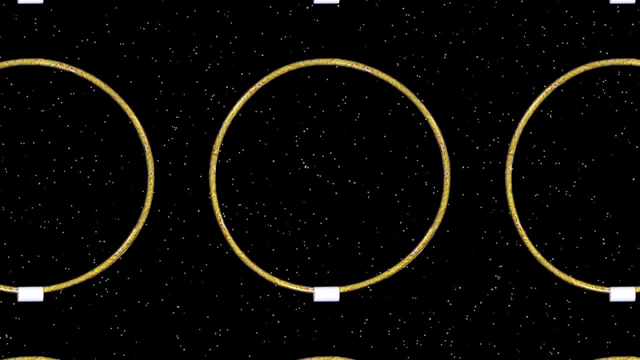 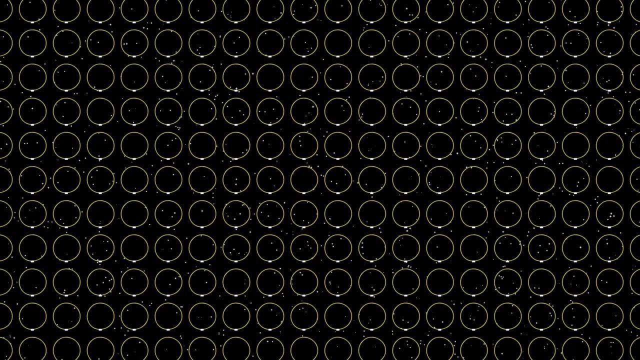 Now imagine that the hula hoop is small, so small that you can't see it. The location of the hoop still needs three dimensions to describe it, but there is still the question of where the paper is. To answer that question, you need four dimensions. 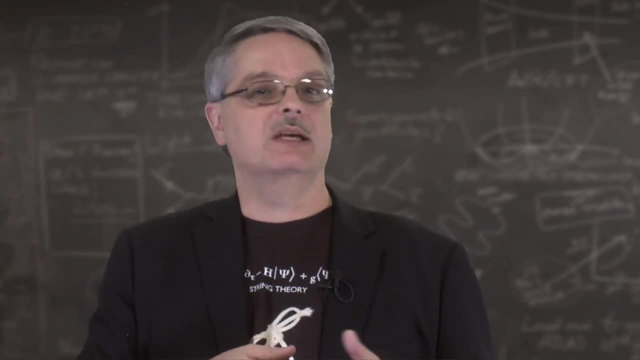 Now I know that some of you will say that it's a little bit too big for the paper. but no, no, no, You can't do that. I will say that as I move the paper around the loop, it is also moving in the ordinary. 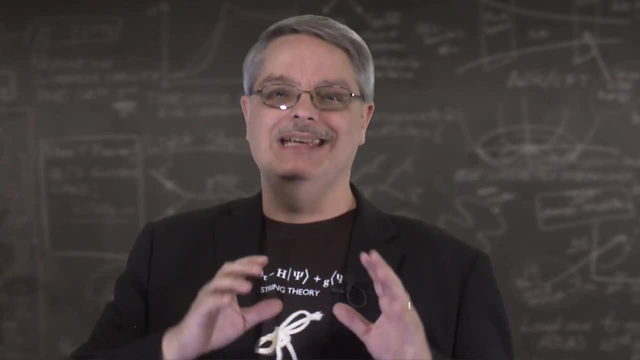 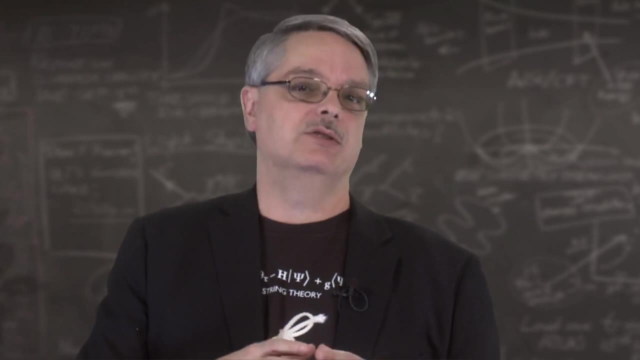 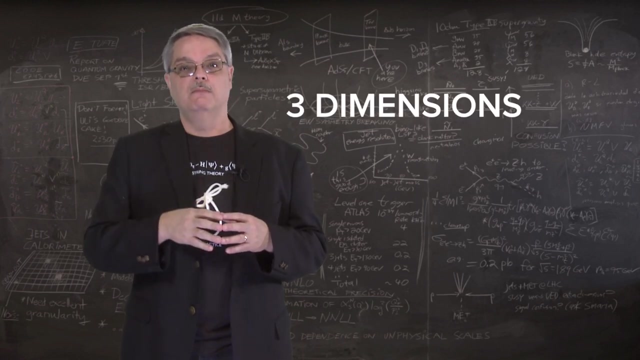 three dimensions. And you're right. Just remember I'm using an analogy to describe a very complex mathematical idea. The analogy is imperfect, but I hope it conveys the right idea. So in superstrings you need three spatial dimensions of x, y and z, plus the dimension. 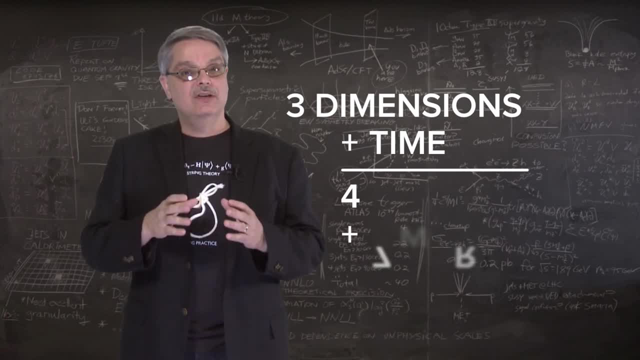 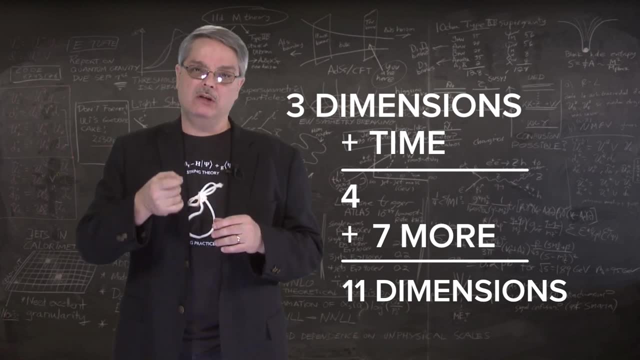 of time That makes four, But you also need seven small extra dimensions, making a total of eleven. Pretty mind blowing, to be sure, but if you just remember a small string vibrating in seven dimensions, you get a decent idea of what the theory predicts. 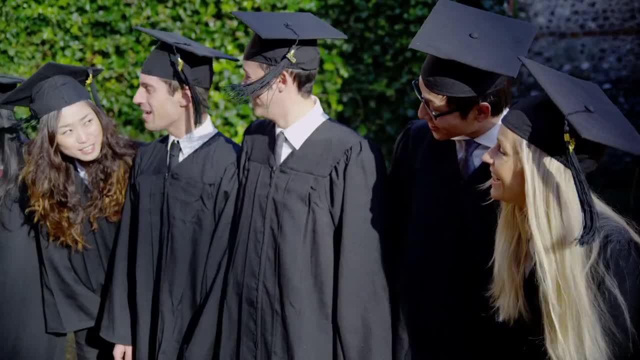 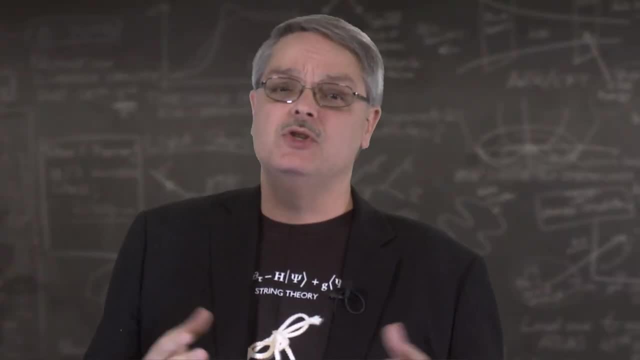 If you want to understand at a deeper level, I have four words for you. Go to grad school. A very important question should be on your mind: Are superstrings real? Should I believe in them? The answer is clear and unequivocal. 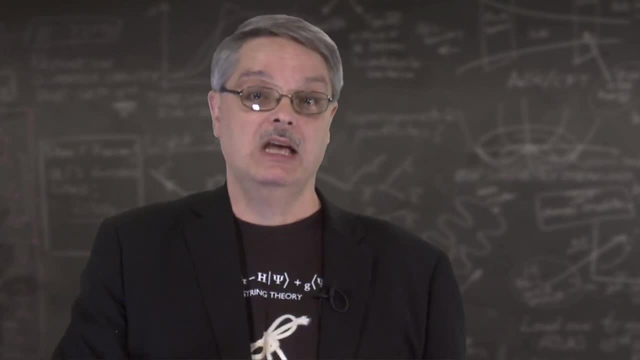 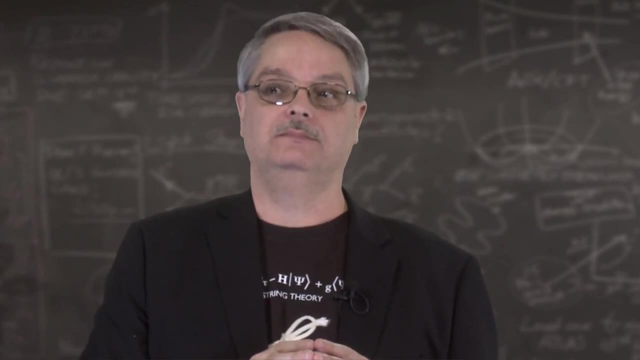 Superstrings might be real, but you absolutely should not believe in them. Superstrings might be real, but you absolutely should not believe in them. They are currently a very cool mathematical idea and there is exactly zero experimental evidence to support them. The reason is simple. 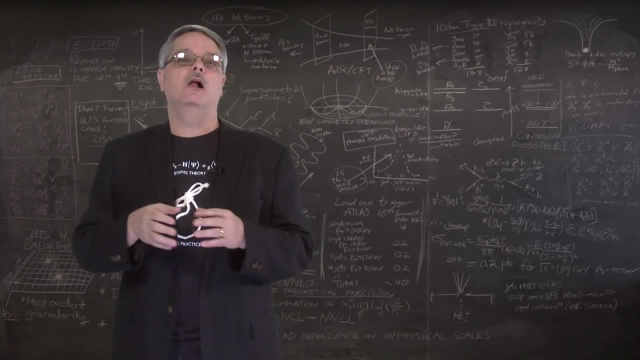 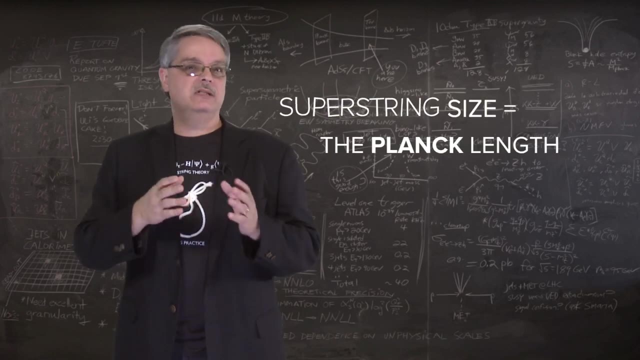 The extra dimensions of superstring theory are incredibly small, much smaller than we can access using our particle accelerators. Physicists imagine that the size of strings might be the Planck length, which is about 10 to the minus 35 meters. That's far smaller compared to a proton than a proton is compared to you. There is no accelerator built, or even imagined, that can explore such tiny sizes. So why do scientists study this idea that is so hard to prove? Well, first, the idea is just plain cool. 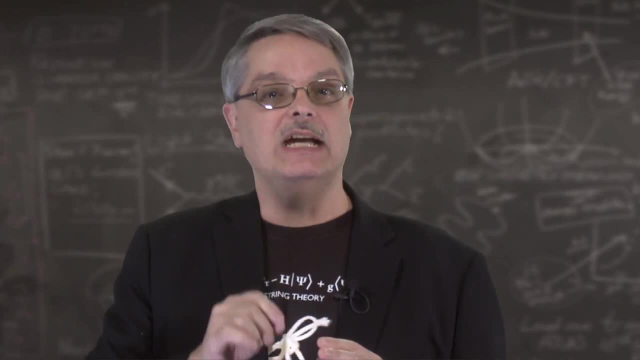 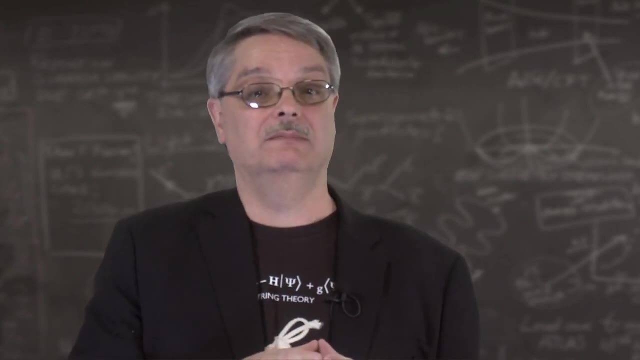 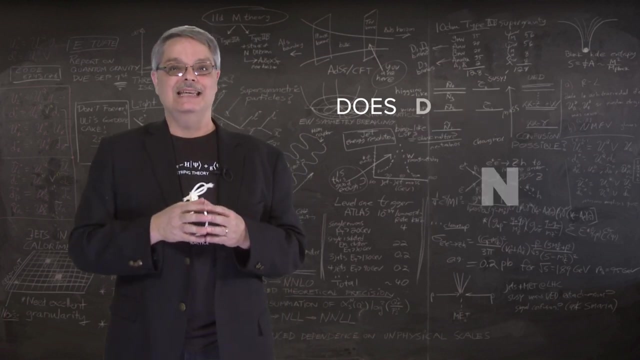 But second, it's a nice and simplifying explanation that finally gives us a simple and fundamental building block that can then explain the complex world we actually live in. When people ask me if I believe in superstrings, I have to say no, But I'd like to. 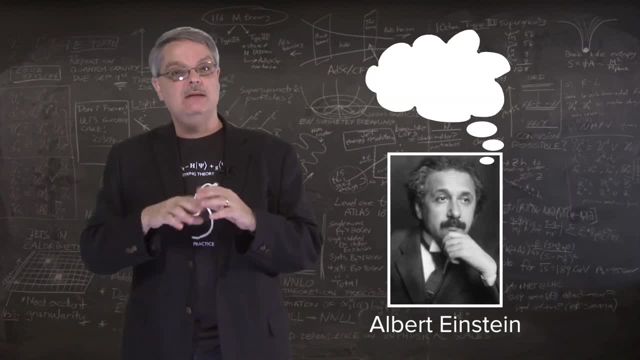 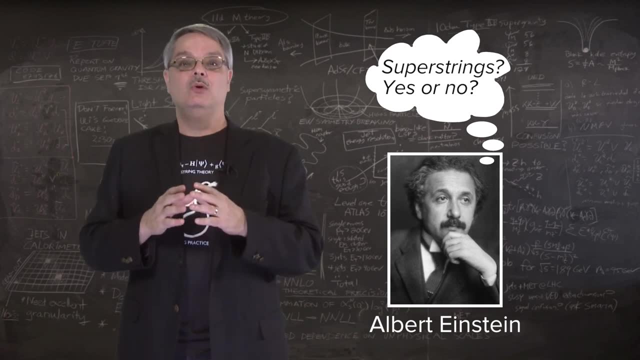 The idea is intriguing and compelling, and I want theoretical physicists to keep thinking about the idea. Maybe they will eventually come up with a way to experimentally verify the model, And then we'll know if superstrings are really a brilliant explanation or just another. 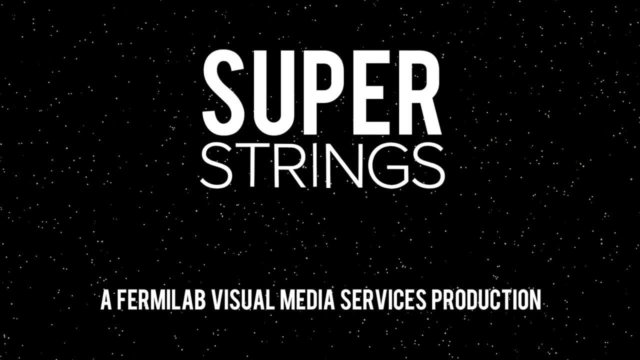 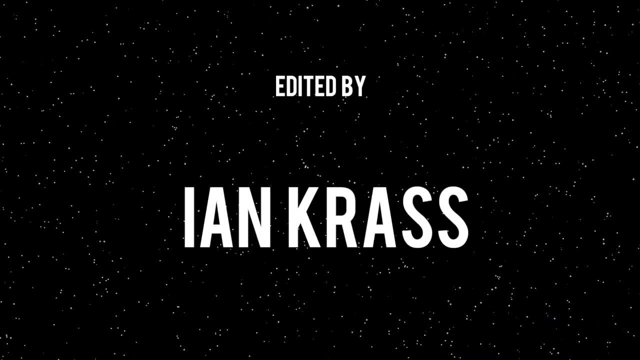 idea that didn't work. Subtitles by the Amaraorg community.